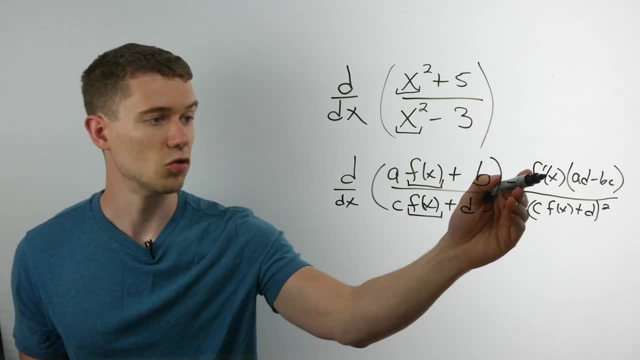 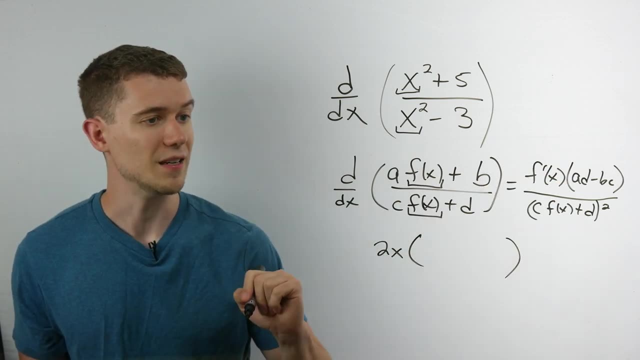 the derivative of the action function, and then that sums all this. so we can just plug it in and we can just of x squared, which is f of x. in this case, The derivative of x squared is 2x. And then it's times: ad minus bc. 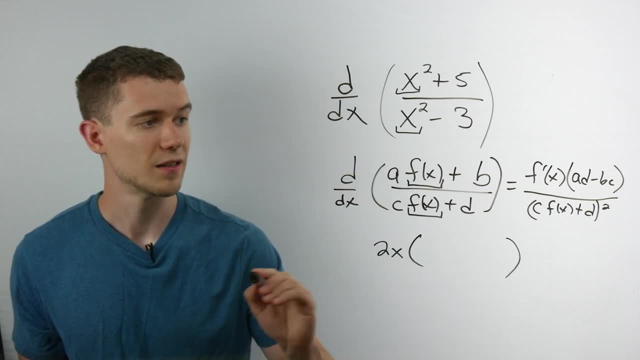 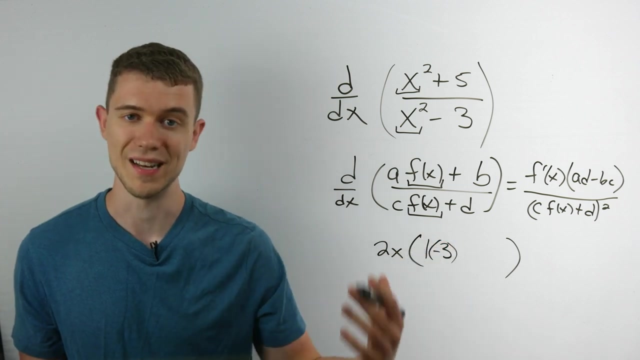 So a is in front of this first f of x, So that's simply 1 in our case. times d. Well, in this case, our d is 3.. In fact, it's minus 3.. Got to be careful with the negatives. 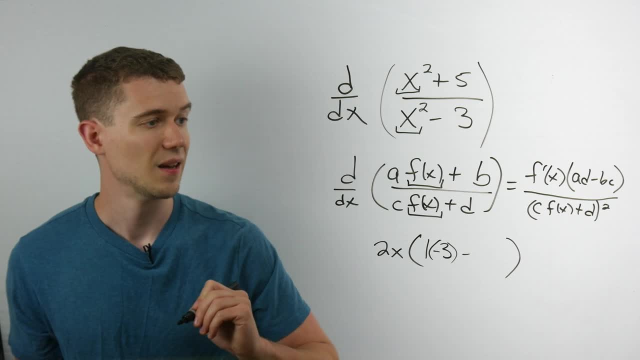 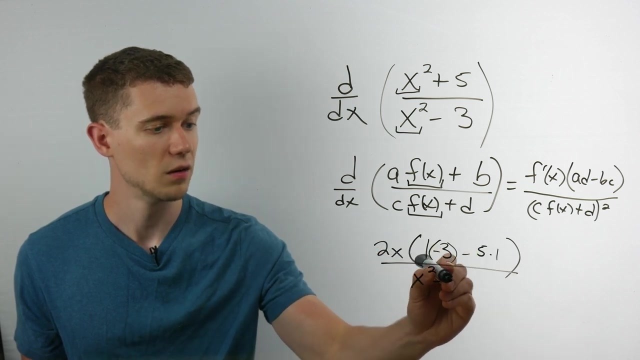 Those also apply here, Minus b, which in this case is 5, times c, c in this case is 1, the coefficient of this f of x, And then that's all over the denominator squared. And so if you simplify this, we'll. 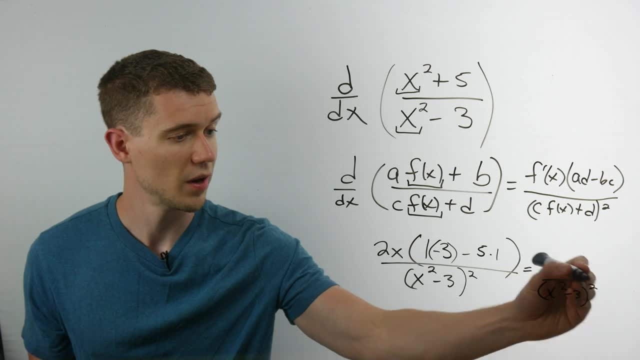 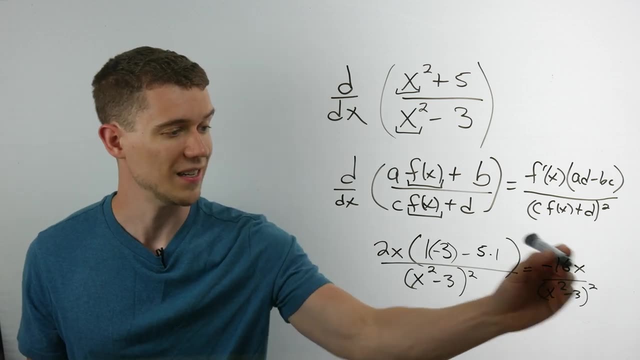 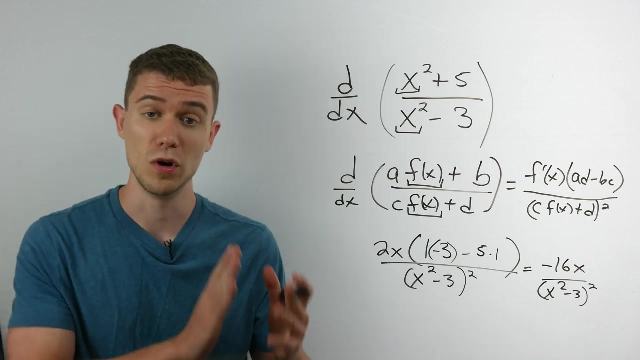 simply get the bottom squared. I'll have minus 3. minus 5 is negative 8. Times 2 will give me that negative 16x on top. And there you go. It's all nice and done. Let me show you another good example. 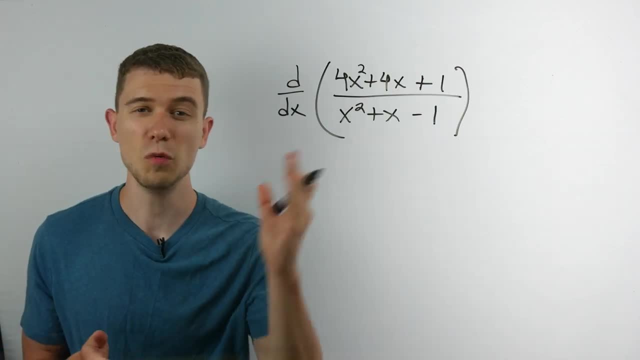 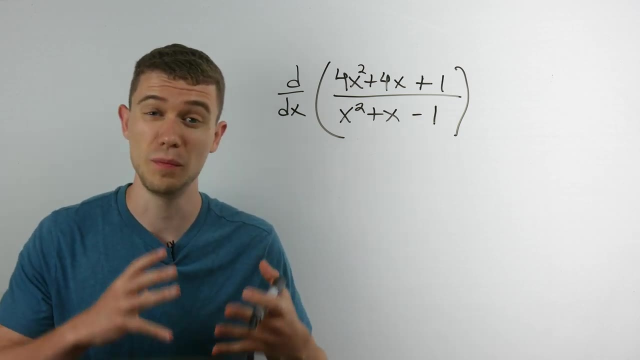 where you can use this trick that you might not have expected. I want to take the derivative of this function, But if I were to use the quotient rule to simplify it, then it would be a little bit messy, It would be a little bit annoying. 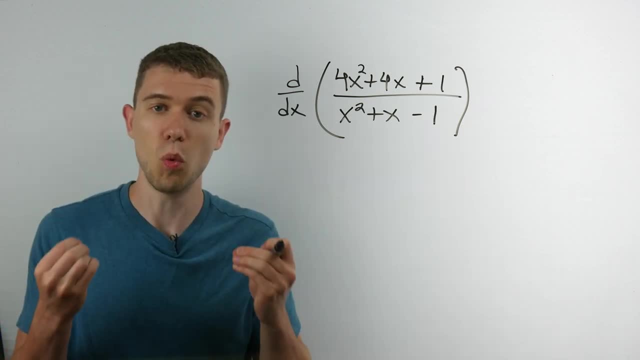 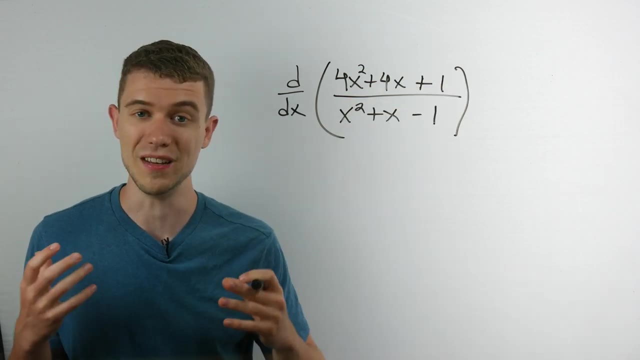 So I'd love to use my trick, But my trick requires that the first two functions on the top and the bottom be the same and the last two be constants. Well, ah, they're not quite the same in this case, Or are they? 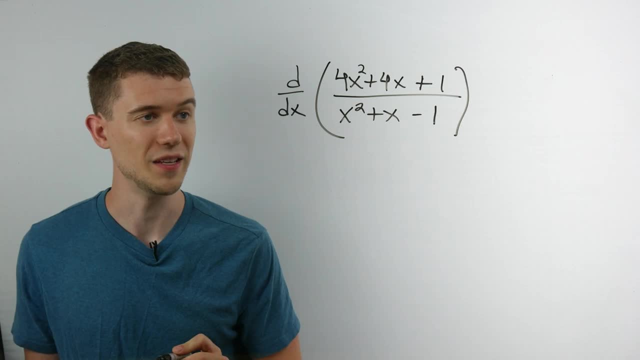 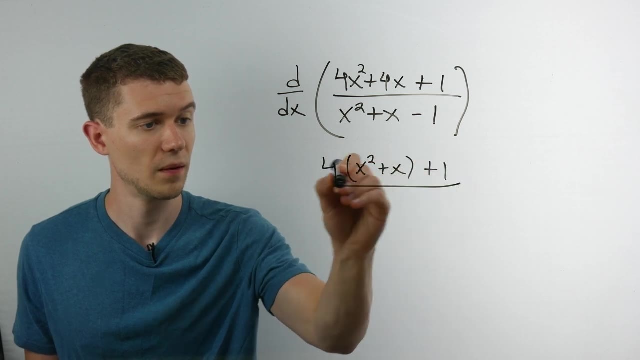 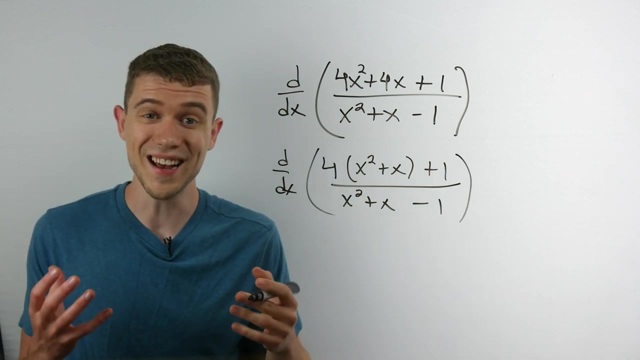 You'll notice, here there's a factor of 4 in common between the x squared and the x term. What if I factor that out? Well, all of a sudden now we're able to use the trick, Because the first two functions match. 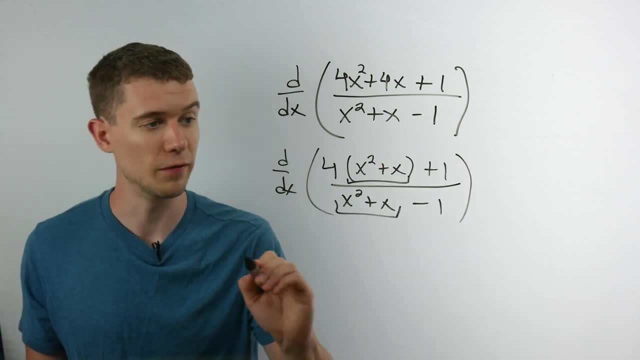 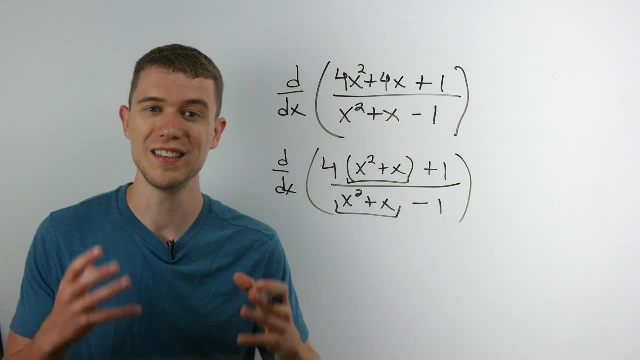 And they're followed by constants. Here, my a will be 4., My b will be 1., My c will be 1. And my d will be 1., In fact, negative 1.. So let's just plug this in to the formula trick.